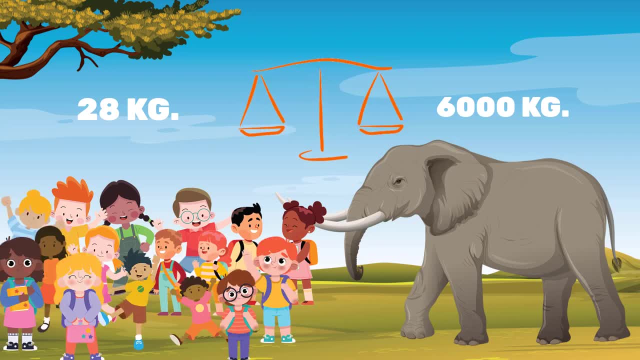 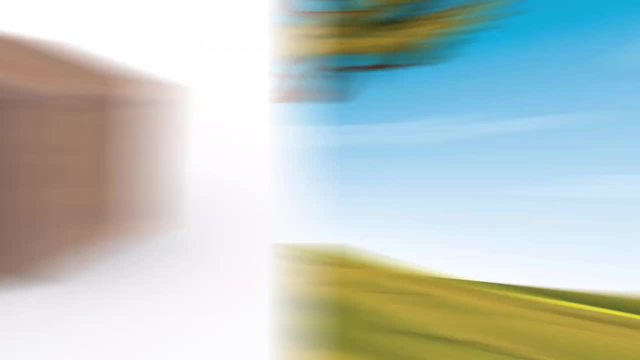 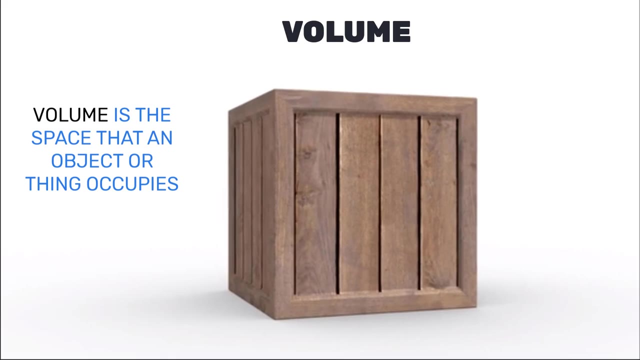 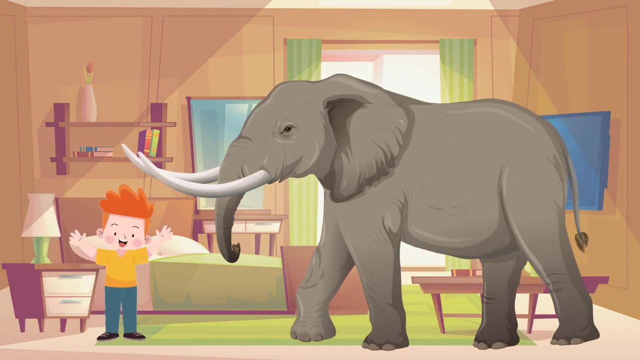 almost two kilograms. two hundred and fifteen children to weigh the same as an elephant- Wow, Awesome, right Another property of matter is volume, which is the space that an object or thing occupies. For example, if you put the elephant and the child in the same room. 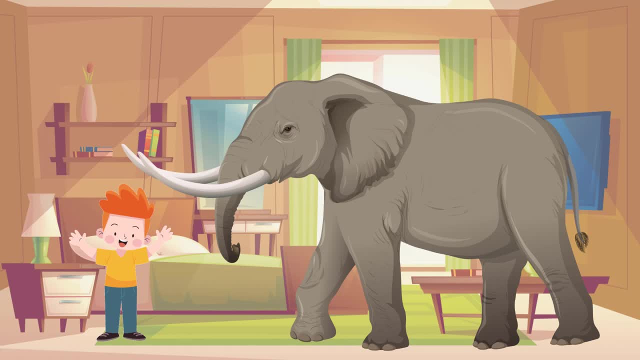 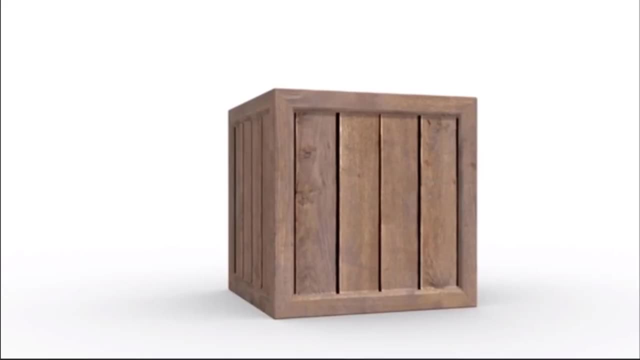 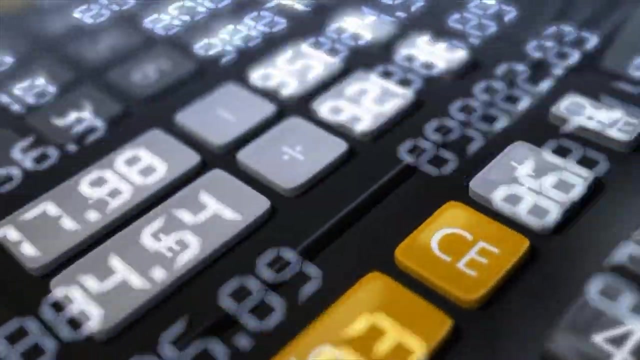 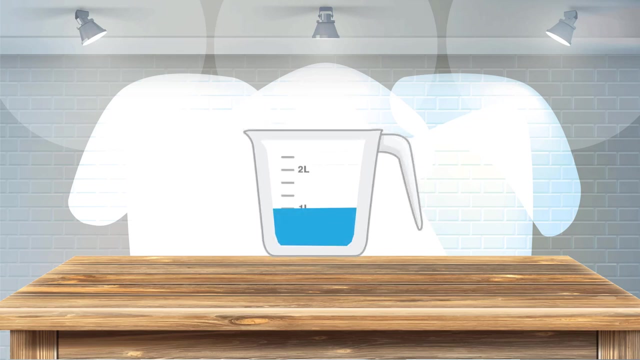 we see that the elephant occupies more space than the child, so its volume is greater. The volume is measured in cubic metres or litres, and to calculate it in a simple way with small objects, you can use a measuring glass and fill it up to, for example, one litre. 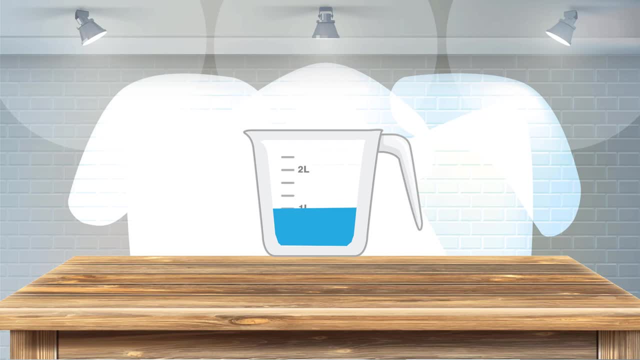 And in this you slowly, slowly drop the object whose volume you want to know, In my case a ball. You will see that the ball will make the water rise. so the volume of the ball will be the difference between the measure of the water with the ball. 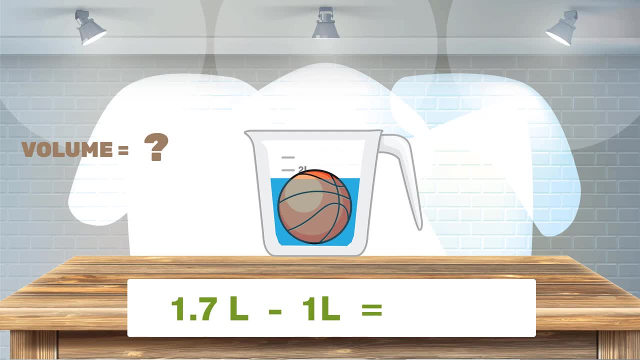 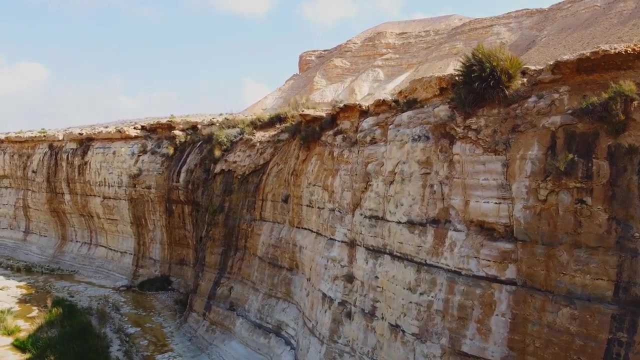 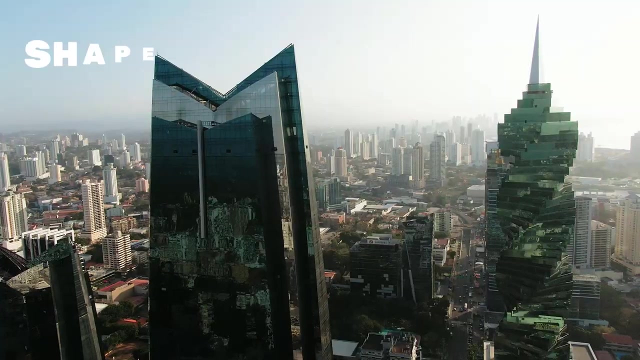 minus the measure of the water without the ball, So the volume of the ball is 0.7 litres. super cool. Other properties are the characteristics which allow us to differentiate one matter from another, such as colour, shape, elasticity, density. 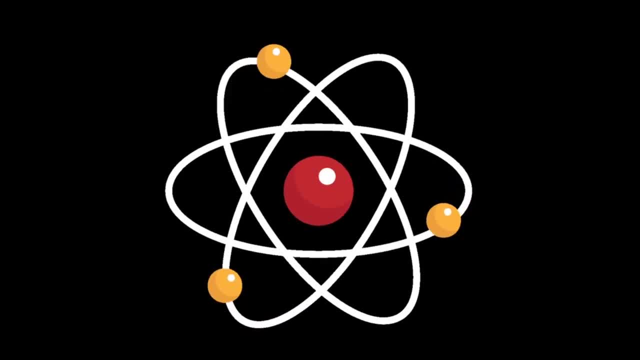 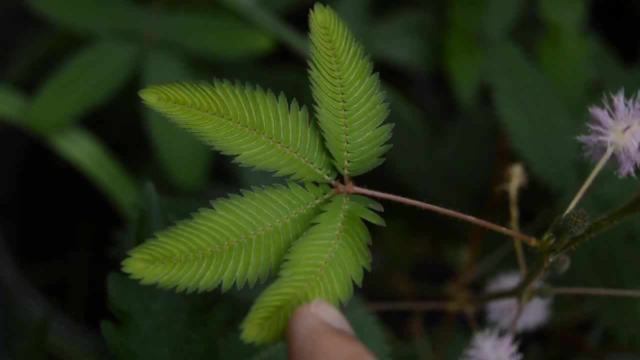 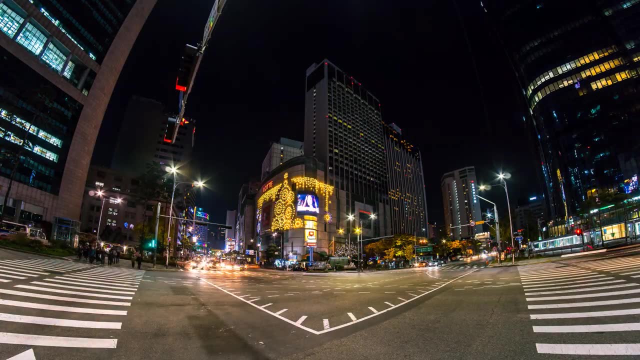 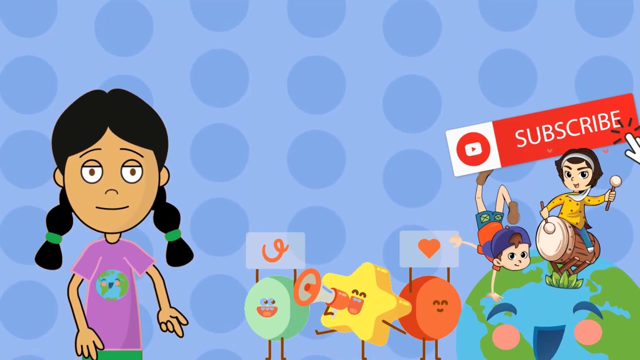 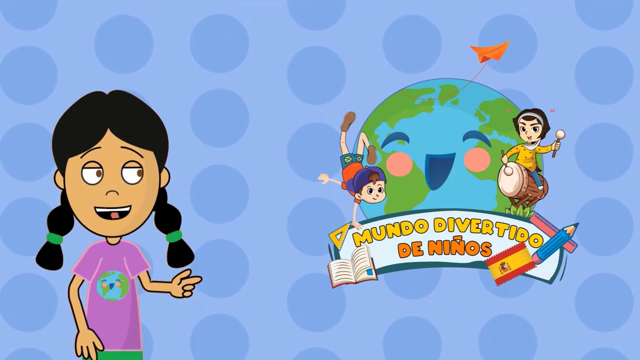 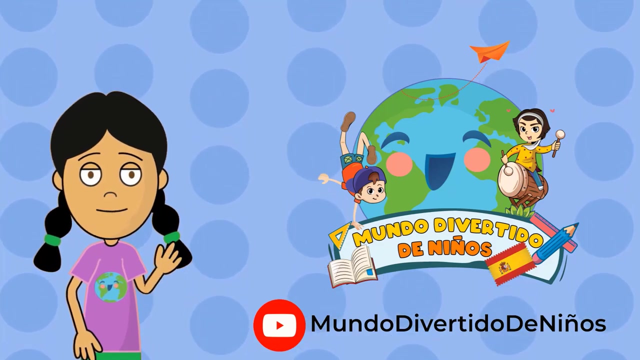 among others. So, guys, each subject has its own characteristics, and it is through the knowledge of its properties that we can know and relate to each subject and, in general, to the world that surrounds us. Lots of love, Bye, bye.